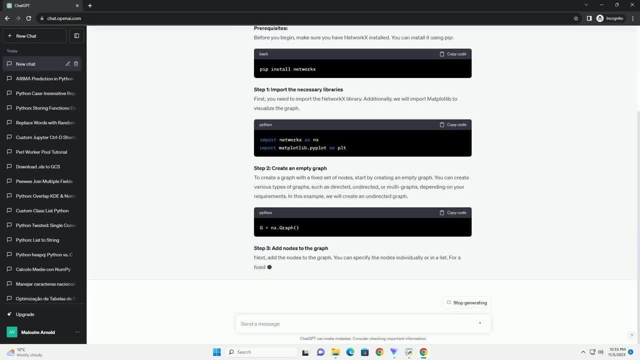 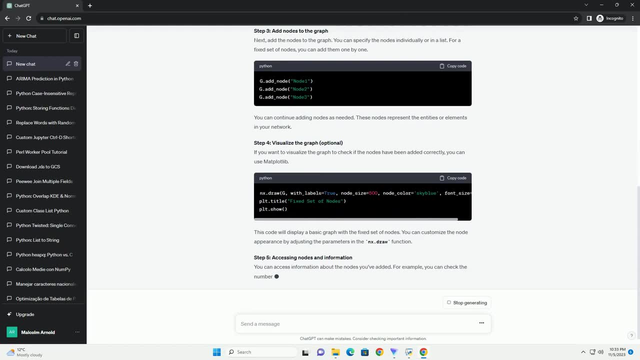 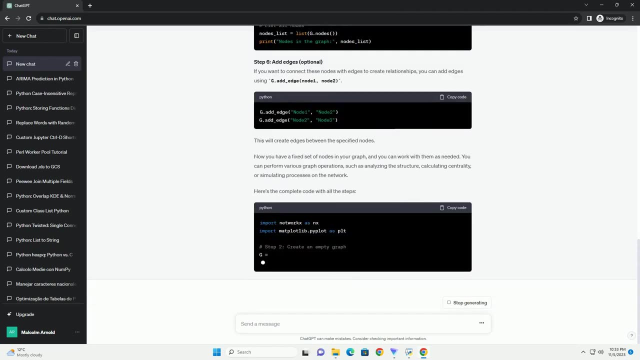 We'll cover the basics of creating nodes, adding them to a graph and setting their attributes. You'll also see code examples to help you understand the process. Step 1. Installation. If you haven't already installed NetworkX, you can do so using pip. 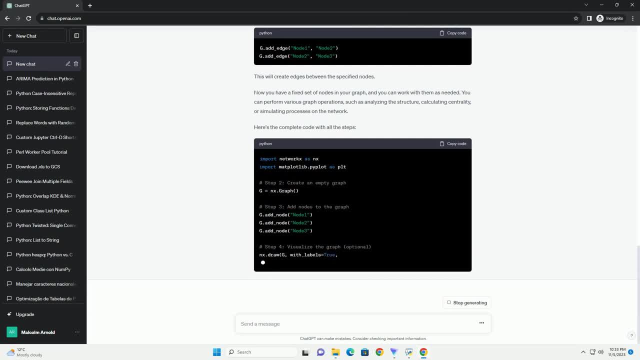 Step 2. Import NetworkX. Begin by importing NetworkX into your Python script or Jupyter notebook. Step 3. Create an empty graph. You can create an empty graph by selecting the appropriate graph type. For this tutorial, we'll use an indirect graph. 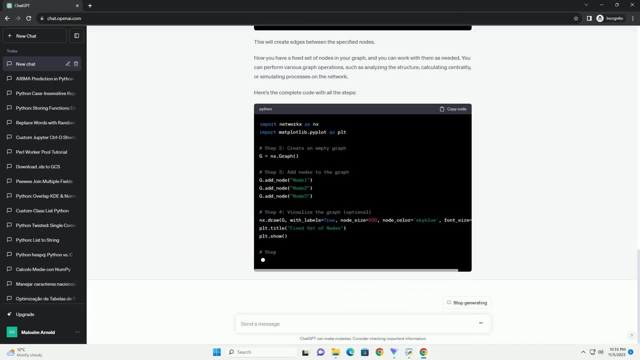 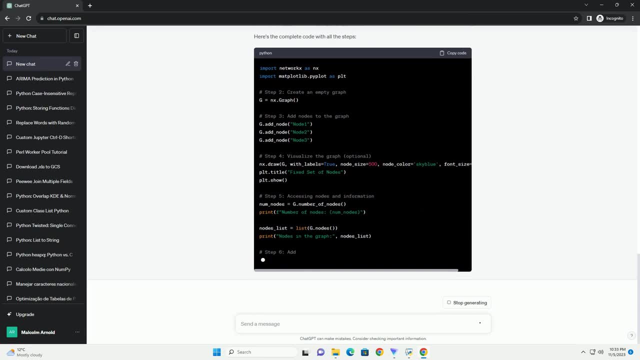 To create a graph, use the following code: Step 4. Adding nodes to the graph. To create a fixed set of nodes, you can add nodes one by one or pass a list of nodes to the graph. Here's how to add nodes to the graph. 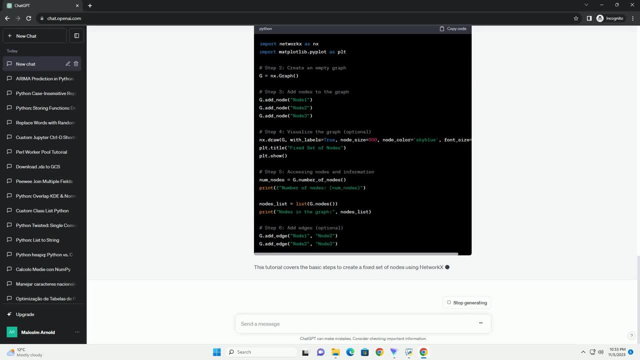 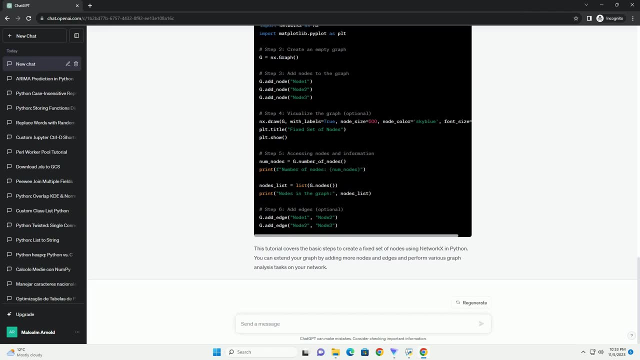 Now you have a graph G with nodes A, B, C, D, E and F. Step 5. Setting node attributes. You can assign attributes to nodes which can be useful for storing additional information about each node. Here's how to set node attributes. 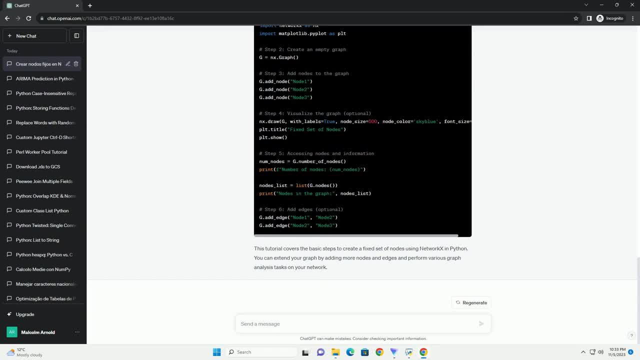 Now nodes A, B and C have attributes: color and size. Step 6. Visualizing the graph. You can visualize your graph using NetworkX and other visualizing tools. You can visualize your graph using NetworkX and other visualizing tools. 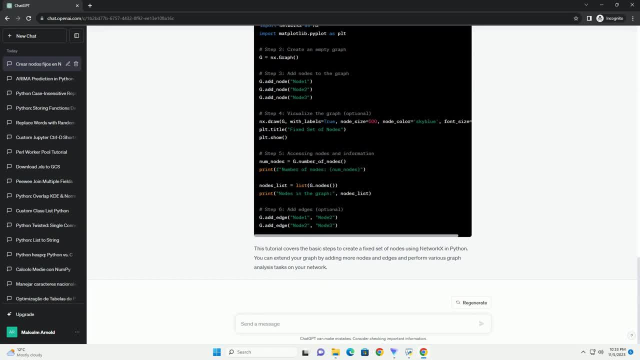 Step 7.. Adding attributes to the graph- Step 8. Adding attributes to the graph. You can add objects and other visualization libraries like Matplotlib. If you haven't installed Matplotlib, you can do so with. Here's an example of how to visualize your graph. 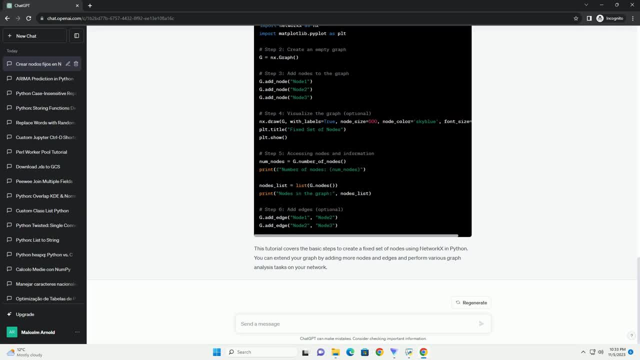 Here's an example of how to visualize your graph. This code will create a simple visualization of your graph, with nodes colored and sized based on their attributes. That's it: You've learned how to create a fixed set of nodes using NetworkX in Python. You can now manipulate and analyze your network. add edges, organization nodes, etc. You can now manipulate and analyze your network, add edges, organization nodes, etc. You've learned how to create a fixed set of nodes using NetworkX in Python. 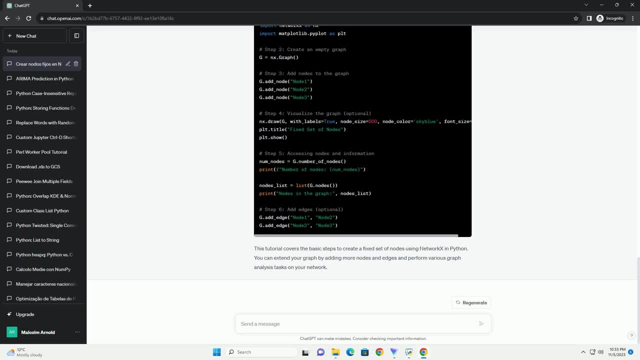 add edges and perform various graph operations based on your specific requirements. Chat, GPT. Creating a fixed set of nodes using NetworkX in Python is a common task when working with network graphs. NetworkX is a powerful library for creating, analyzing and manipulating complex 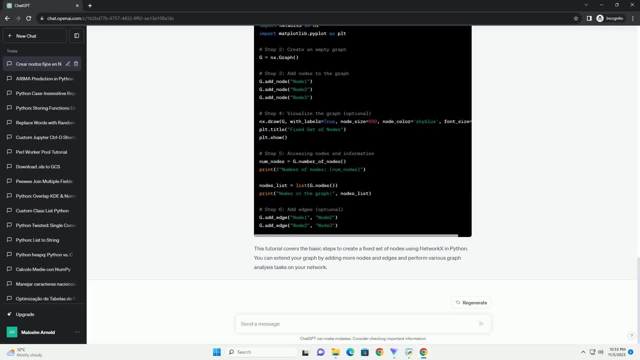 networks and it offers various functionalities to work with nodes and edges. In this tutorial we will walk through the steps to create a fixed set of nodes in NetworkX and provide code examples to demonstrate the process. Prerequisites: Before you begin, make sure you have NetworkX installed. You can install it using PIP. 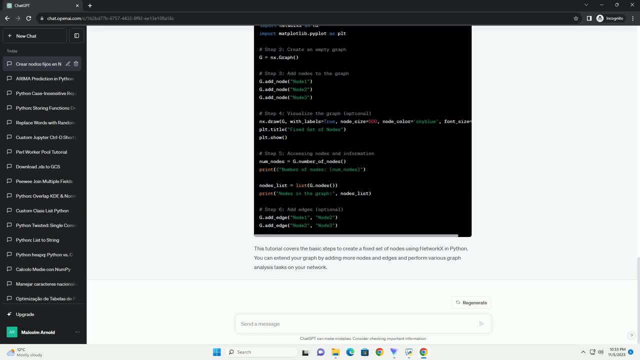 Step 1, Import the Necessary Libraries. First, you need to import the NetworkX library. Additionally, we will import matplotlib. Step 2, Create an Empty Graph. To create a graph with a fixed set of nodes, start by creating an empty graph. You can. 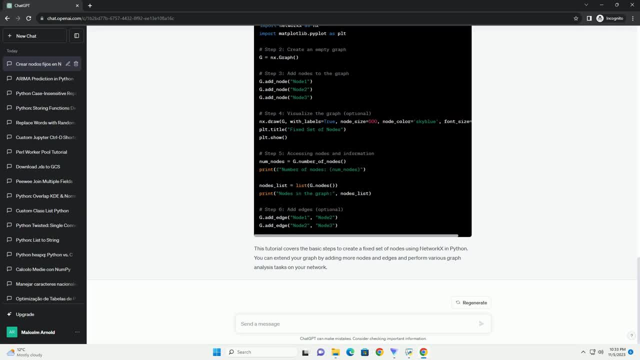 create various types of graphs, such as directed, indirect or multi-graphs, depending on your requirements. In this example, we will create an indirect graph. Step 3, Add Nodes to the Graph. Step 3, Add Nodes to the Graph. 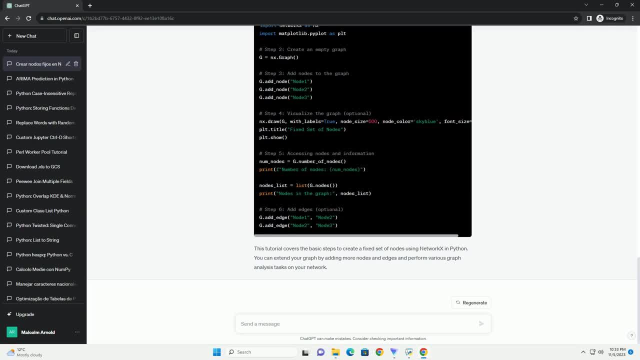 Next, add the nodes to the graph. You can specify the nodes individually or in a list For a fixed set of nodes. you can add them one by one. You can continue adding nodes as needed. These nodes represent the entities or elements in your network. 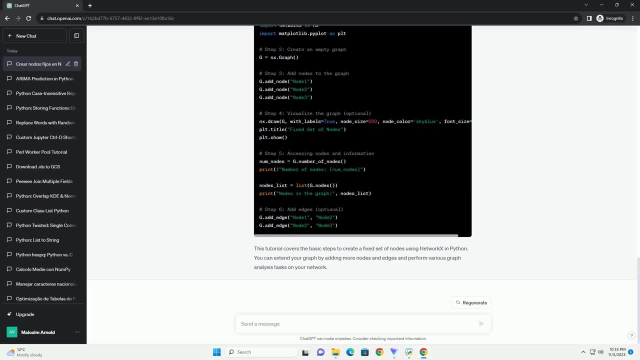 Step 4, Visualize the Graph. If you want to visualize the graph, to check if the nodes have been added correctly, you can use matplotlib. This code will display a basic graph with the fixed set of nodes. You can customize the node appearance by adjusting the parameters in the nxdraw function. 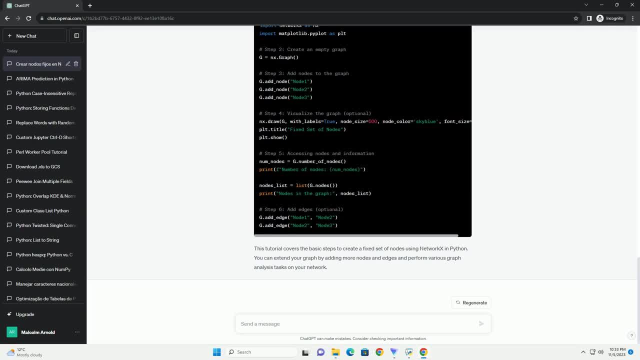 Step 5, Accessing Nodes and Information. You can access information about the nodes you've added. For example, you can check the number of nodes and list all the nodes in the graph. Step 6, Add Edges. If you want to connect these nodes with edges to create relationships, you can add edges. 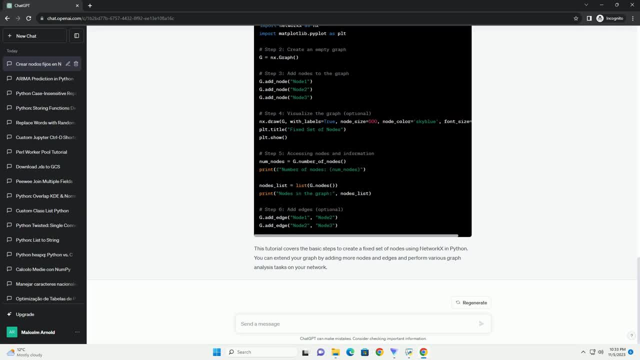 using gadd__edge. This will create edges between the specified nodes. Now you have a fixed set of nodes in your graph and you can work with them as needed. You can perform various graph operations, such as analyzing the structure, calculating centrality or simulation. 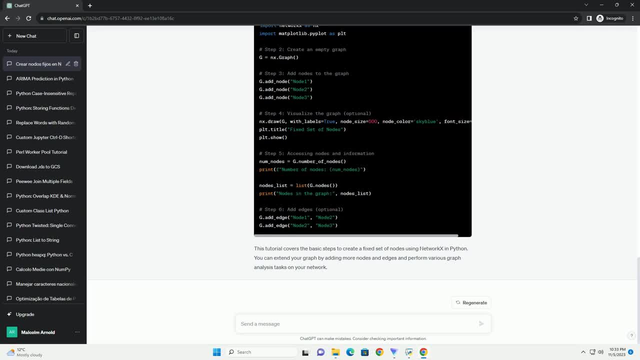 Here's the complete code with all the steps. This tutorial covers the basic steps to create a fixed set of nodes using NetworkX in Python. You can extend your graph by adding more nodes and edges and perform various graph analysis tasks on your network, ChatGPT. 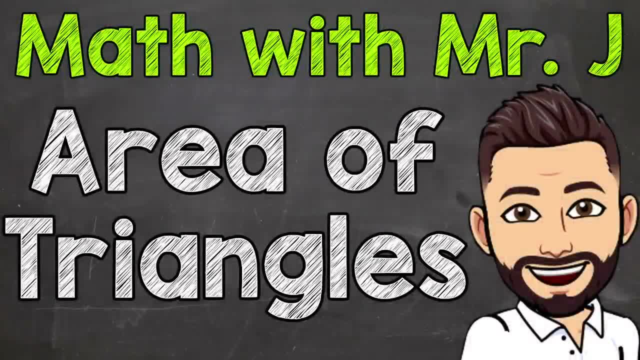 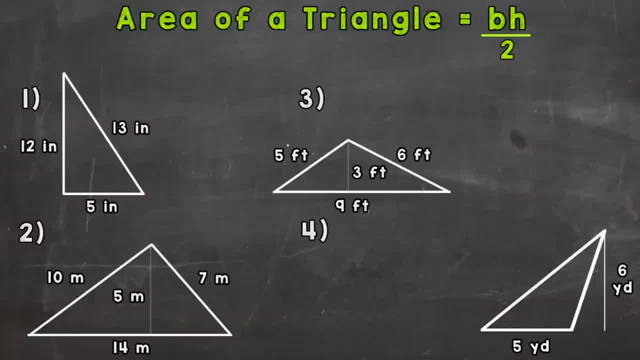 Welcome to Math with Mr J. In this video I am going to cover how to calculate the area of a triangle, And remember area is the amount of space a two-dimensional or flat shape takes up. Our formula for finding area of triangles is at the top of your screen: BH divided by 2, and that means base. 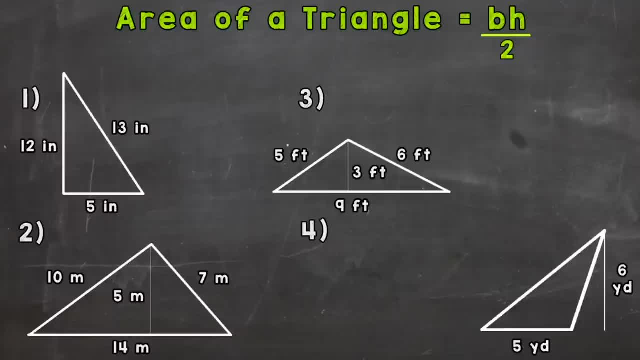 times the height divided by 2. And that's going to give us the area of the triangles on your screen, or any triangle that you are finding the area of. So, like I just mentioned, you have some problems on your screen and you have four of them. 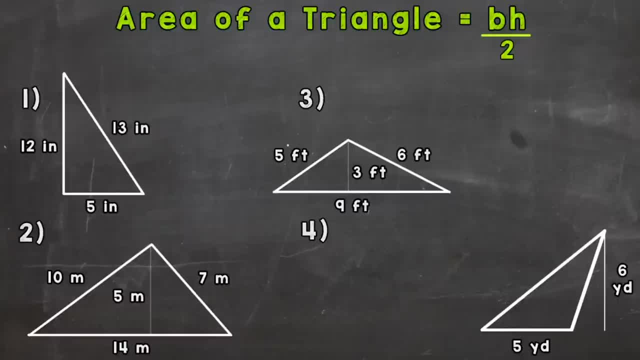 that we are going to work through together. So let's hop right in to number one. So for number one here, the first thing we want to do is write out our formula for the area of the triangle. So what we're going to do is we're going to